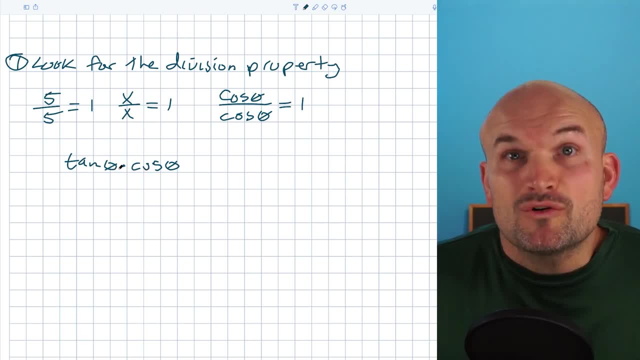 here right, There's no division property. So if I want to look for or create the division property, one thing I can do is I can rewrite tangent as a sine of theta over a cosine of theta. Now you can see that I have a cosine of theta in the numerator and a cosine of theta in the. 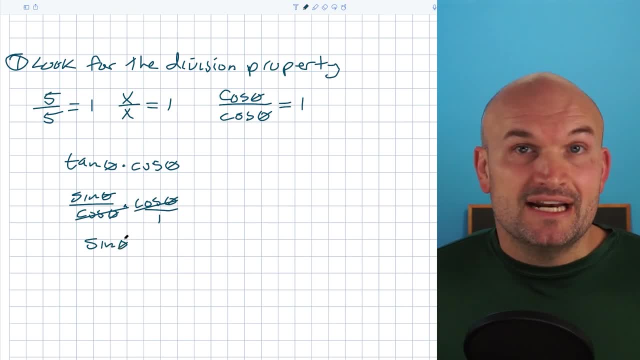 denominator. So therefore, these are now going to divide out into a sine of theta. Now, a mistake that students will make sometimes is they, instead of rewriting tangent as a sine over cosine, they'll maybe go ahead and rewrite tangent as a sine over cosine. They'll maybe go ahead and 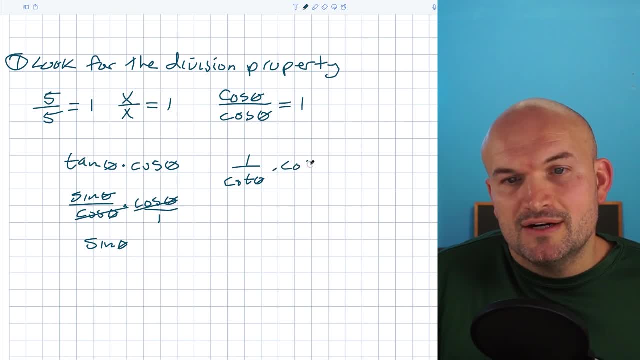 rewrite it as a one over a cotangent of theta. Well, you can see here that does not help us with the division property. When you're looking for the division property, you want to look for the same term in the numerator as well as in the denominator that is going to divide out. It's. 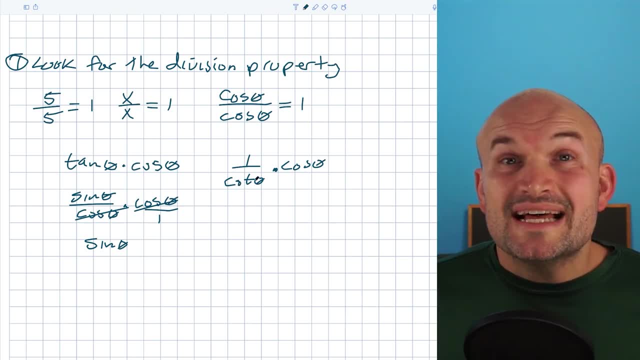 also important sometimes to not always oversimplify the problem. So that's the main thing: when you're simplifying these expressions, especially when you're dealing with a rational expression, look to apply the division property, Look to simplify or rewrite your terms. So therefore, 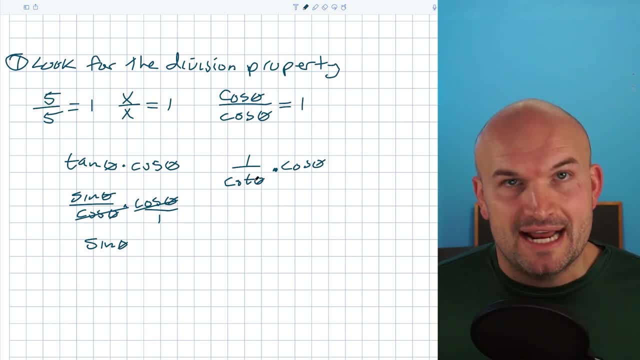 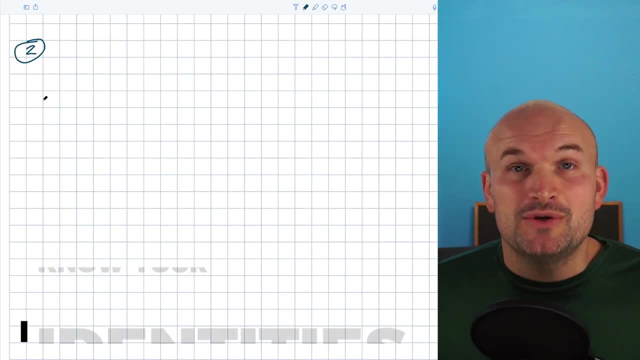 you can have the same term in the numerator and denominator that you can divide out. And remember the division property can be applied across multiplication but not addition and subtraction. Tip number two is you have to know your identities. I'm talking about the Pythagorean identities. 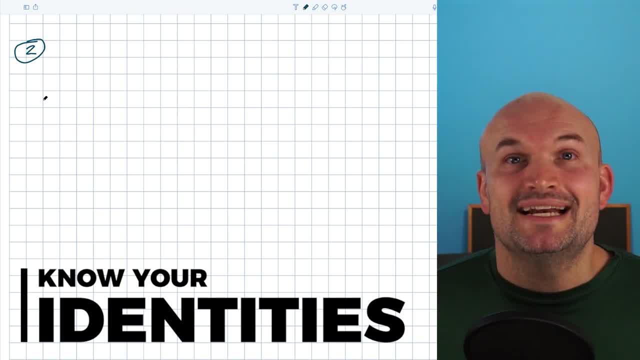 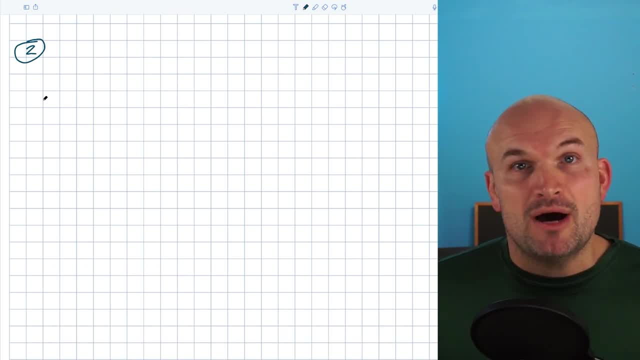 the co-function identities, the even odd identities, the reciprocal identities and the quotient identities. Yes, with practice these will become easier, but it's so important to keep practicing these and know them off the top of your head because, as you're simplifying expressions or verifying identities, which comes next? 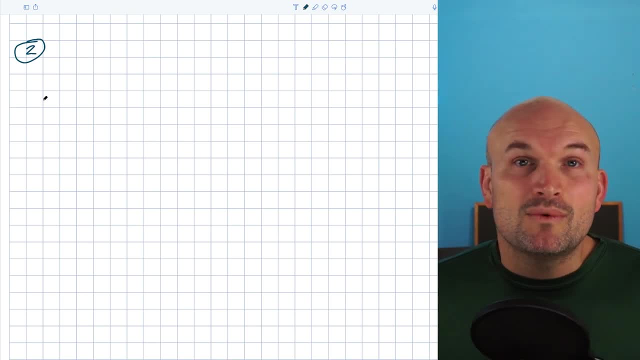 you're going to have to rely on knowing these identities. These are what's going to help make simplifying your trigonometric expressions easy to understand. And yes, I know there's many, many more identities that we could also include on here, but to keep this video simple, 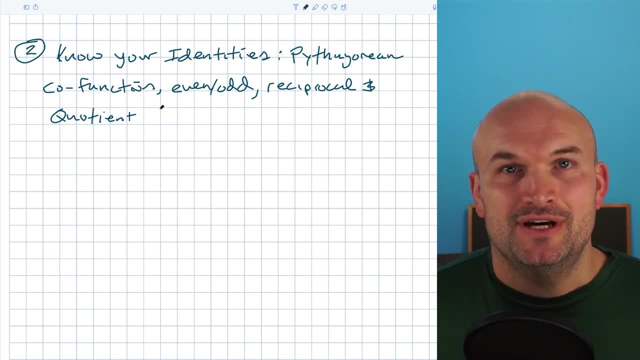 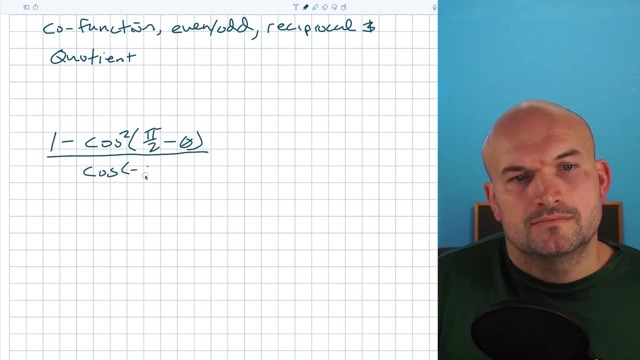 I'm just going to focus on these basic identities that you have to make sure you know, All right. so let's go and take a look at an example that can look very, very confusing unless you know your identities, All right. so there's a couple of ways that students get confused here. 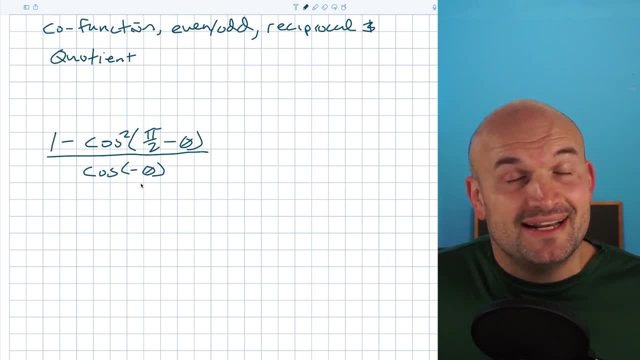 Whenever we see a pi half minus theta, that's confusing, The cosine of negative theta. a lot of students forget that, And then also the squared here. students a lot of times kind of forget what exactly that means. So what I'm going to do is just kind of rewrite this expression in: 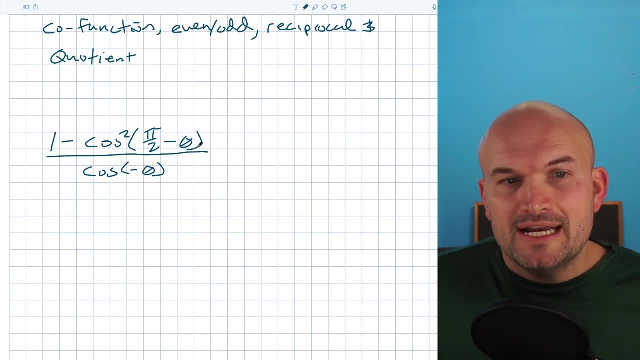 a couple of different ways so we can see the identities clearly and then apply them. Now the first thing I'm going to do is I'm going to rewrite this cosine squared actually as the function squared. So whenever you have cosine theta of pi half minus theta, we can rewrite: 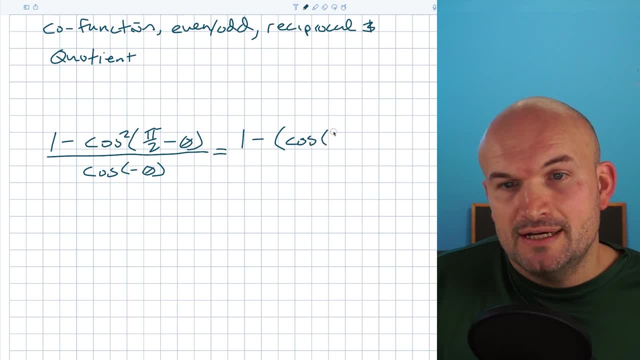 this as a one minus cosine of pi half minus theta quantity squared, And then I'm just going to rewrite the denominator as the same. Now, the reason why this is important: because I want you to know that we don't want to write the denominator as the function squared, We just like to put the 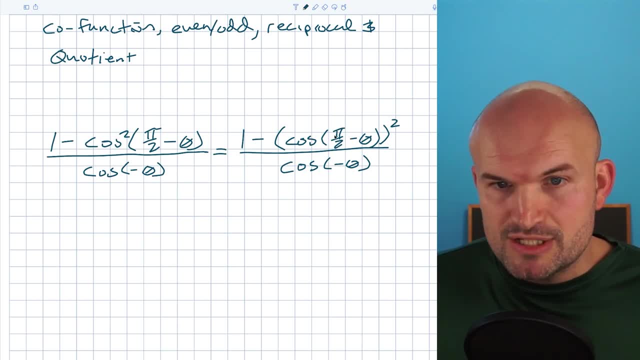 squared here, because we don't want to confuse it with making the argument squared. The reason why this is important to look at this view, though, now, is because you can see that the cosine of pi half minus theta- while that can be confusing sometimes because it looks like a lot's going on- 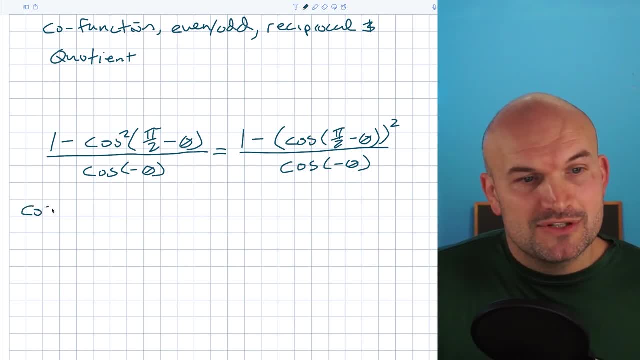 that's actually just our co-function identity that you're going to need to know. So the cosine of pi half minus theta is equal to a sine of theta. And then also we see the cosine of negative theta. Well, that is also another identity, That is your even odd identity. So the cosine of negative theta. 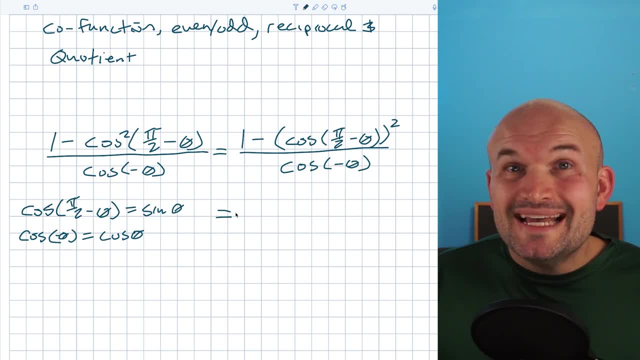 is equal to the cosine of theta. So what's nice about having these identities is now I can just rewrite these as another simplified form. So I can rewrite this as a one minus a sine squared of theta, divided by a cosine of theta. But we're not done yet. If we need to simplify these, we want to keep. 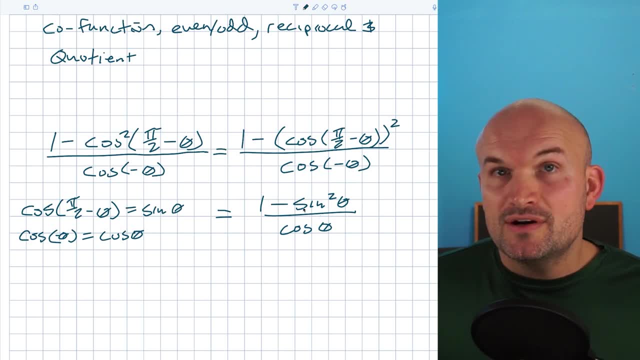 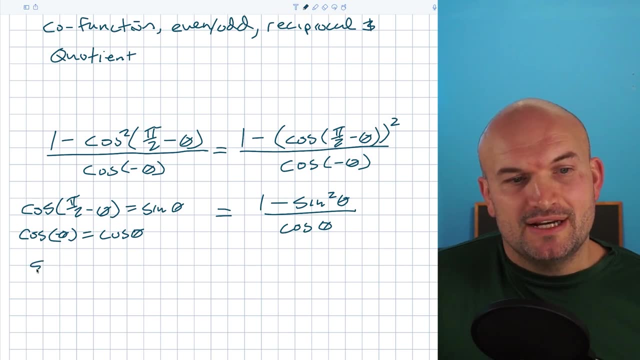 on using as many identities as we possibly can, And the one thing I notice is, whenever you have a squared, always a lot to look to your Pythagorean identities. Remember one of the famous Pythagorean identities? here is a sine squared of theta plus cosine squared of theta is equal to one Now. 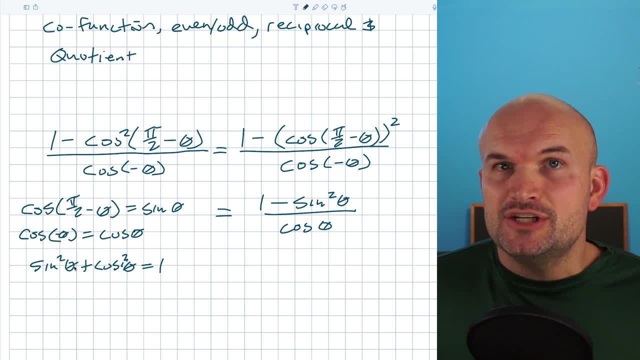 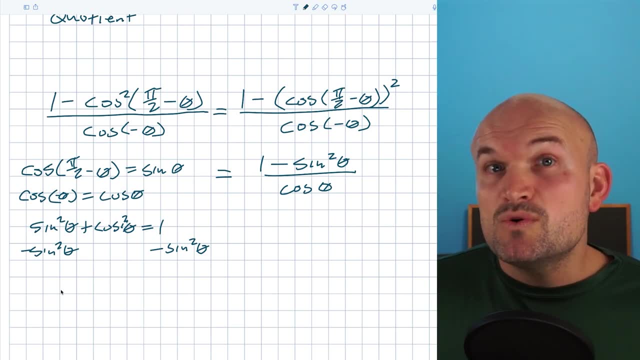 one minus sine squared of theta. out of this expression, all I simply need to do is subtract a sine squared of theta on both sides. Now what that's going to give me is a cosine squared of theta equals one minus sine squared of theta. So what's important about this is now we can take 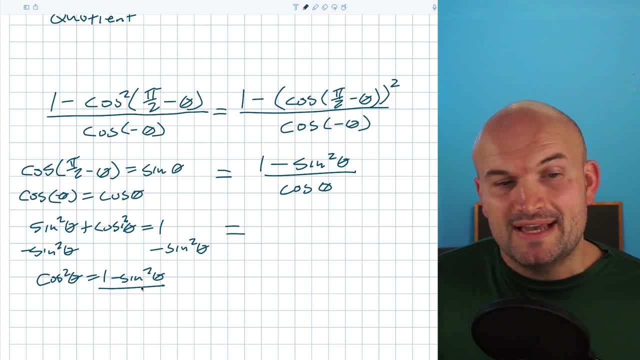 this whole expression and I can replace a one minus sine squared of theta with just a cosine squared of theta divided by a cosine of theta. Now, remember the last tip, when I talked about the division property. we got to be very careful. We got to remember that the cosine squared of theta 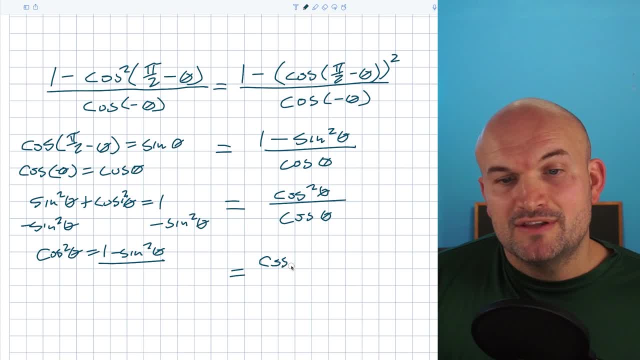 represents the cosine of theta times the cosine of theta. So we have the cosine of theta times cosine of theta divided by a cosine of theta. So again now applying the division property, we can see that we're going to have a final answer. All of this stuff simply just equals the. 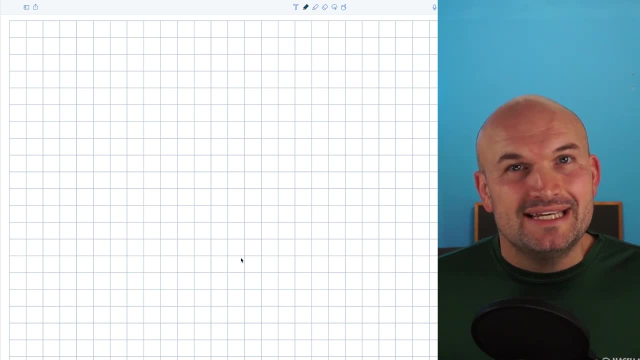 cosine of theta. Now, tip number three is a little controversial. I like to give it to students when they start to struggle with simplifying our expressions, because it's giving them some tools that they're used to. However, I am very hesitant to introduce this to the whole class because some 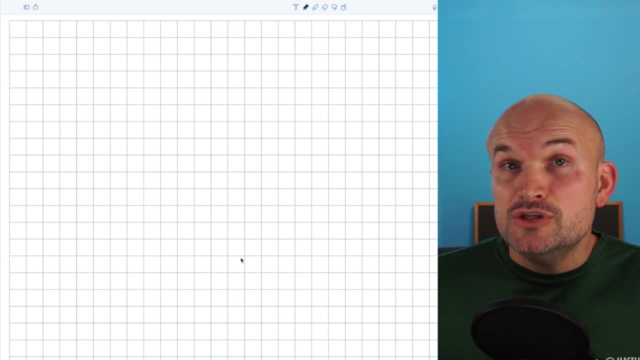 of the things that I'm going to talk about in this video are going to be a little bit more complicated, So I'm going to start off with a little bit of an example of how you can use this as a crutch, And that's not the point that I want you to use this, for. It is a great tool to sometimes when 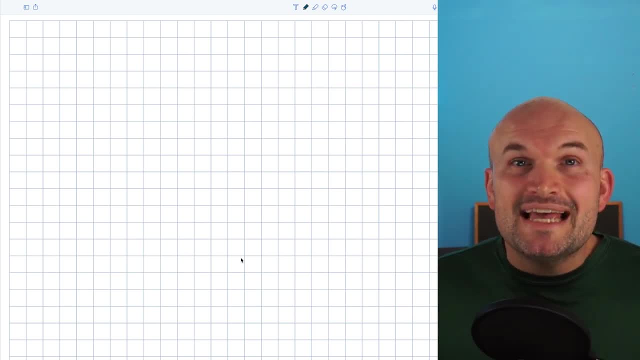 you get stuck or to help you get through something that's a little bit messy algebraically. However, for time's sake as well as for understanding, we're not going to want to do this on every single problem, but it can be very useful to understand, And this tip is simply, rather than: 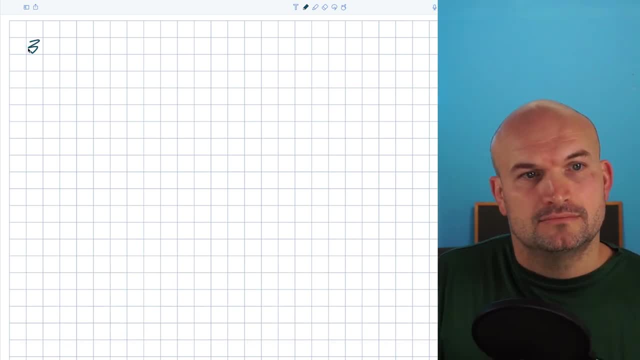 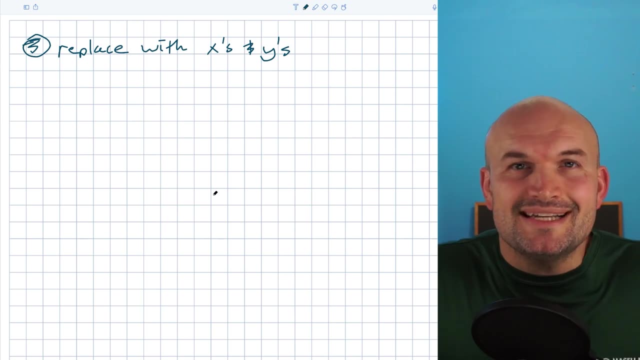 using our trigonometric expressions, which sometimes can kind of feel like a lot of words to write on a piece of paper. You don't really need to replace with X and Y's. You could use A's and B's or elemental P's, It doesn't really matter. Typically I like to use sometimes the X. 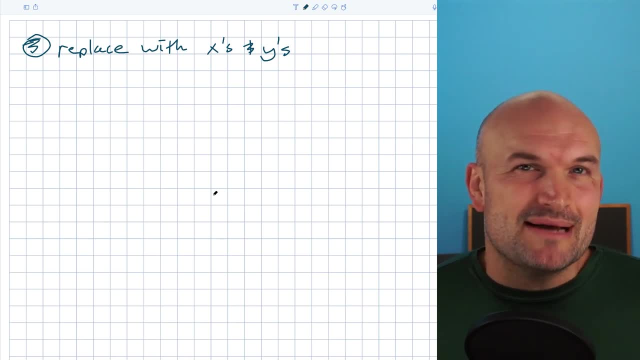 and Y's because those do relate to, like sines and cosines. So sometimes it makes a little sense. And then also algebraically, we're a little bit more used to using X's and Y's to simplify expressions, And a lot of what we're doing with simplifying trigonometric expressions. 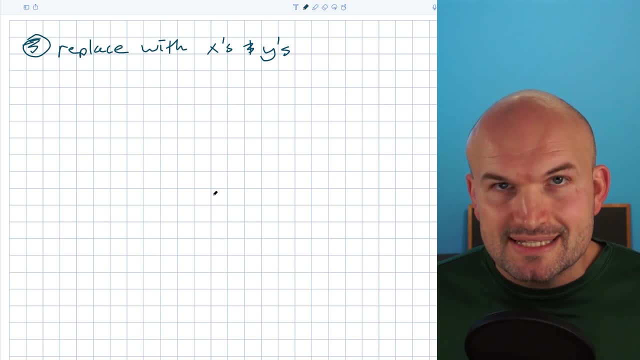 is related to what we did previously with our algebraic concepts. We're applying the same rules, the techniques. It's just now we have some different functions or variables that we're using to apply them. So we're going to start off with a little bit of an example. 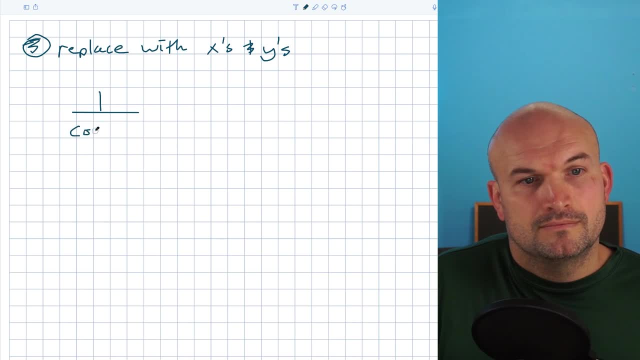 So, for example, when you look at a problem that looks like this, some students will say: I have absolutely no idea how to do that problem. And I'll be like, yes, you do, We've just did this last quarter. And they'll be like, no, I don't know how to do that. 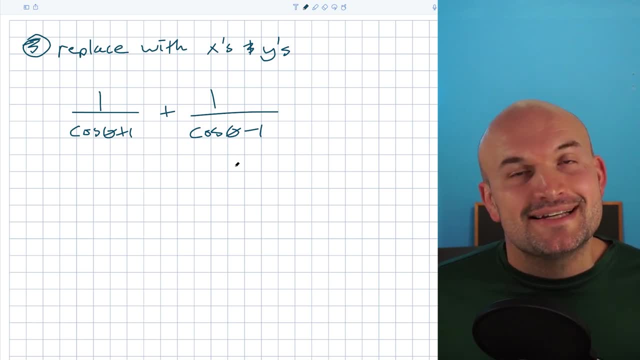 The cosine of theta confuses me, and I don't like fractions And I say: great, Well, why don't we forget about the cosine of theta and let's just use X? Now, this looks like something that we did in our unit on rational functions, And again you could still have problems with how to do this. 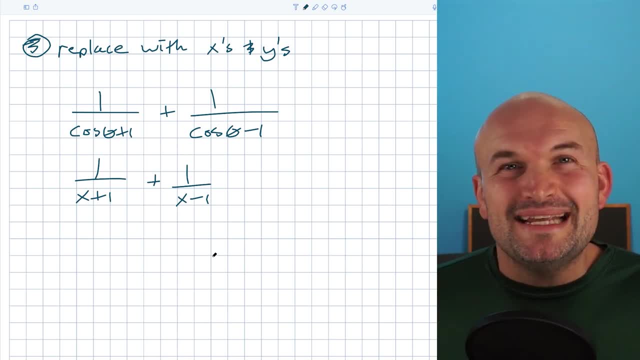 but at least hopefully, it's not going to be a problem. So we're going to start off with a simple formula To help us get to the reality of what's going on. what we need to do is to think about the fact that we're adding in a common denominator, And now we're going to 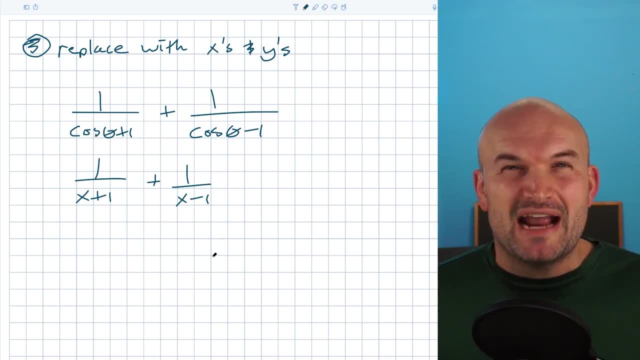 be thinking of how to add in a common denominator. So we're going to look at the common denominator. So what I would recommend is, when you do get stuck, are you having a hard time kind of really kind of understanding how the problem is set up and what to exactly do, what process to look for? 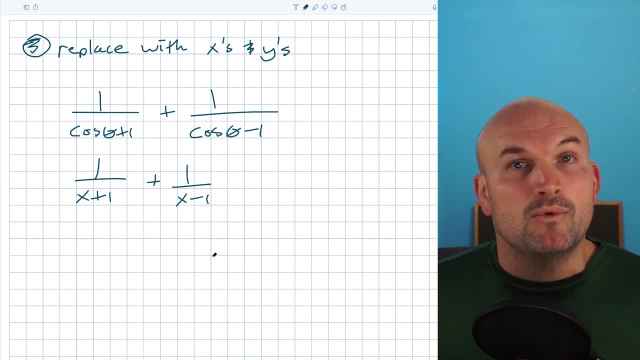 rewriting them in terms of variables sometimes can help unlock your brain on what exactly you need to do. And in this case we need to get a common denominator to add these, because these two fractions do not have a common denominator. So to do that, I'm going to find the common. 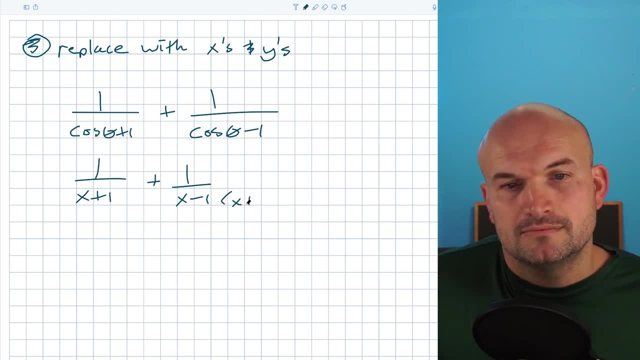 denominator, which is a X plus one times a X minus one. And then now I have a common denominator, I can just go ahead and recombine my two numerators. So you can see, even if we're dealing with cosines, it's going to be the exact same process. 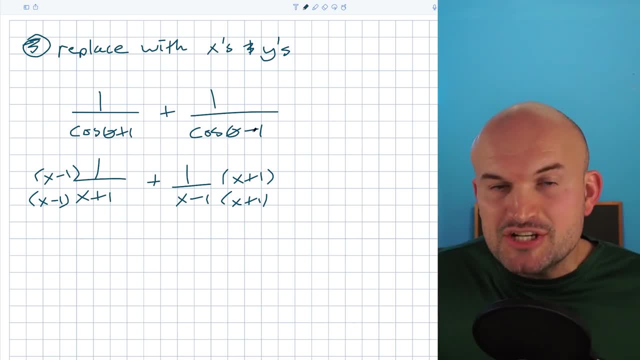 right, We don't have common denominators, but if I multiply by the conjugate, in this case, I can obtain my common denominator. So that's exactly what I'm going to do in this problem. Now I have a common denominator. I can just rewrite this as one single fraction and simplify. 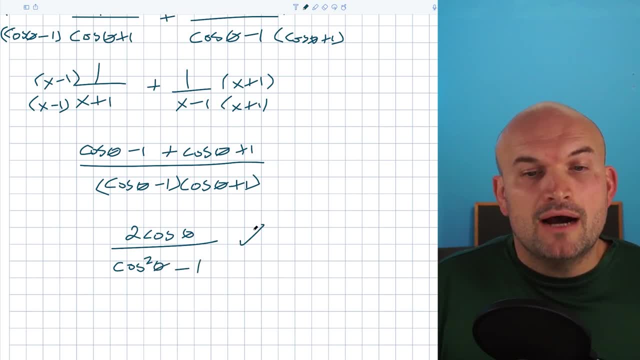 Now we could keep on using our trigonometric identities to simplify this to a negative sine squared of theta, but it's not going to simplify this any further. The main idea that I wanted to talk with you about this is: a lot of students will get stuck. They won't know what to do next. 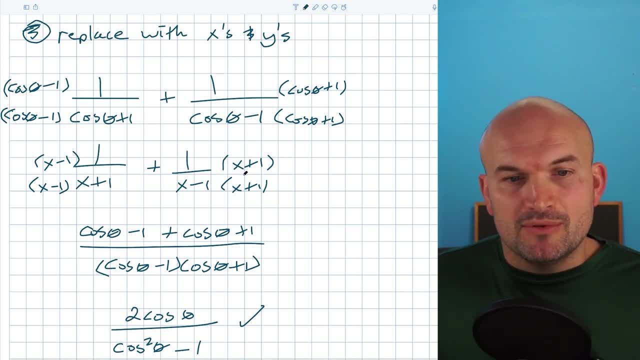 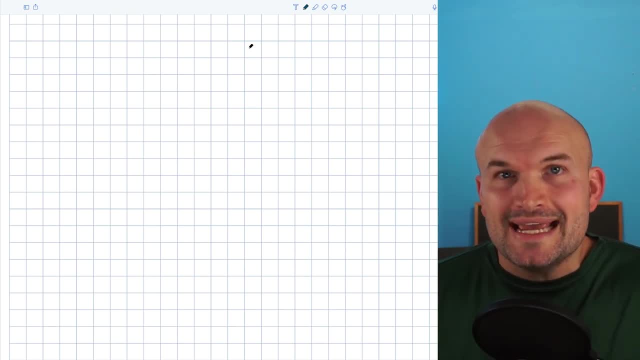 this last tip, using x's and y's, because a lot of times students will relate cosine with x and sine with y And you can therefore rewrite tangent as a y over an x. You can rewrite a cosecant as a one over a y, But, as I mentioned, I don't prefer always using that method because